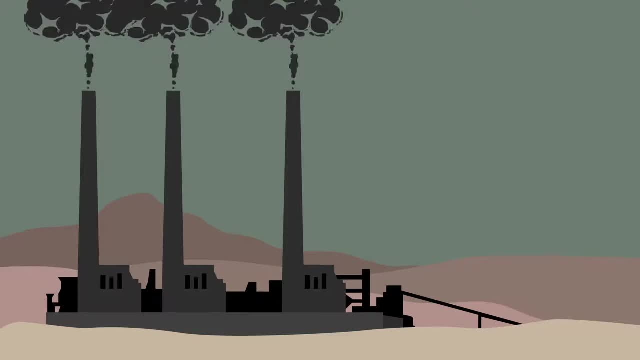 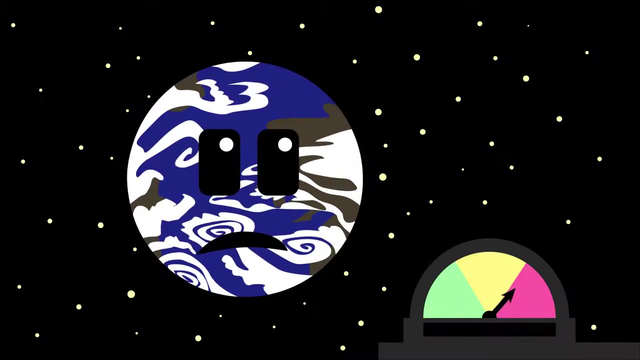 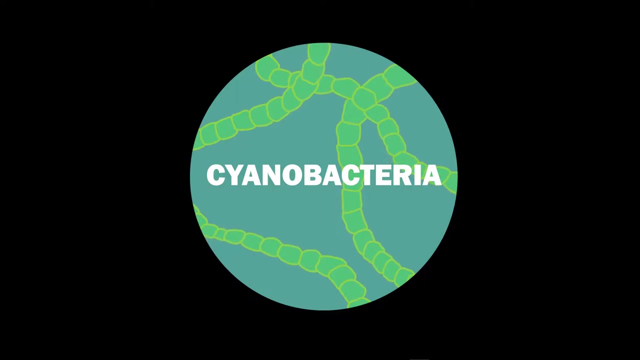 Today we worry about rising CO2 levels. However, it was the buildup of oxygen that caused the first global ecological and climatic catastrophe. The culprit: Cyanobacteria, As the first organisms to evolve the ability to use water in photosynthesis with oxygen. 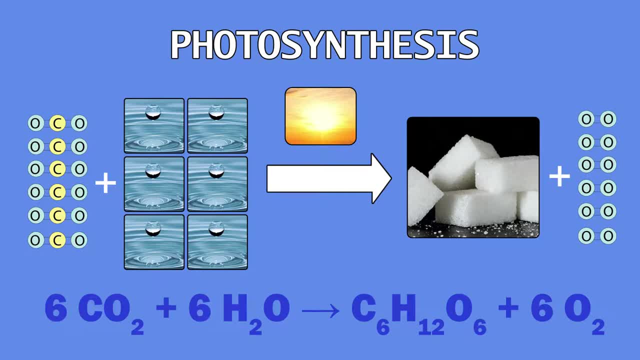 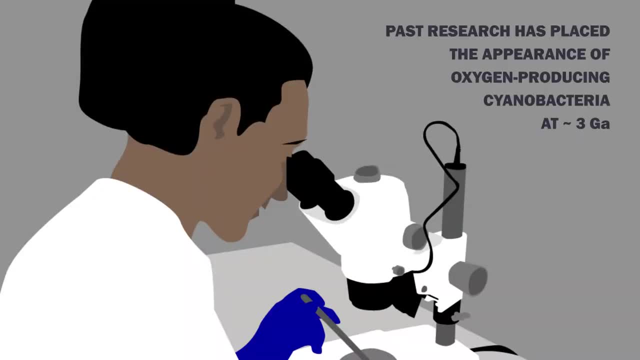 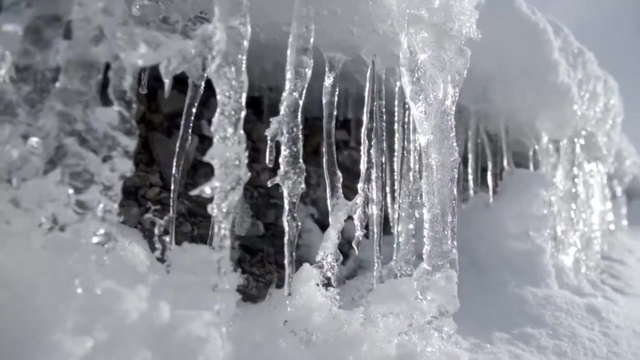 as the waste product. they acquired the ability to grow pretty much anywhere with light and nutrients. Caltech researchers argue that, although past research has placed the appearance of oxygen-producing cyanobacteria at around 3 billion years ago, the first strong evidence for their presence is found around 2.3 billion years ago, immediately preceding the paleoproterozoic. 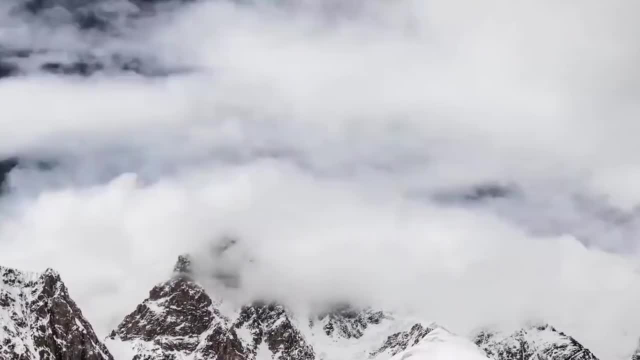 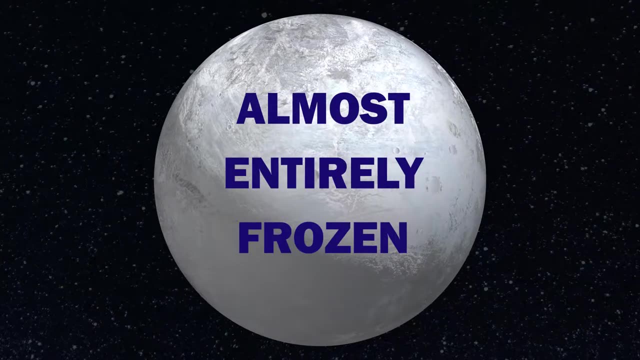 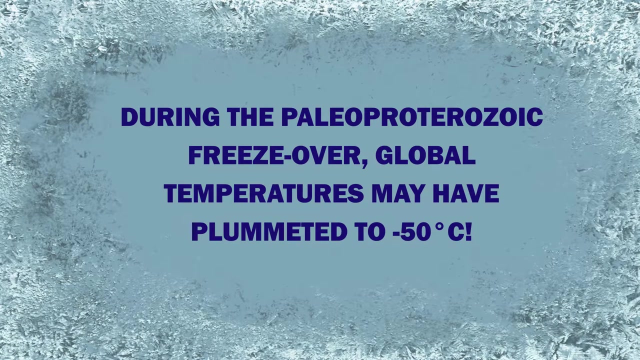 snowball earth. They also argue that the organisms are responsible for this event. During a snowball earth scenario, the earth's surface is almost entirely frozen, and during the paleoproterozoic freezeover, global temperatures may have plummeted to negative 50 degrees Celsius, with even the equator being buried under a mile of ice. 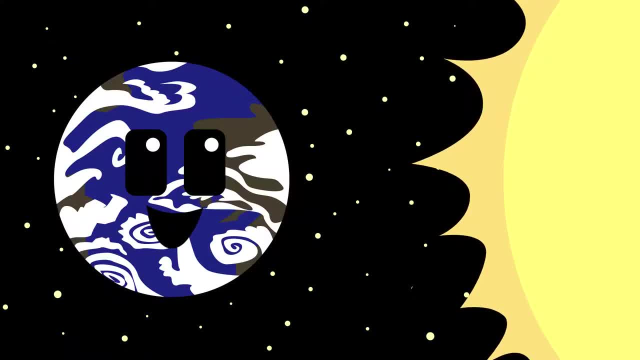 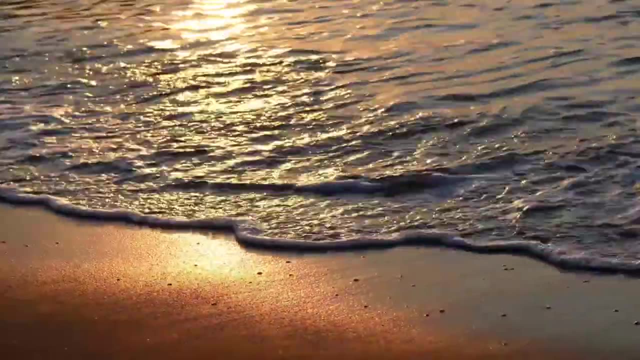 So how was this event triggered? Prior to the extreme glaciation, global temperatures were similar to today's, Although the sun was at only 85% of its current heating capacity. an atmosphere full of methane retained heat. Continental weathering from a series of less extreme glaciations had released large amounts of 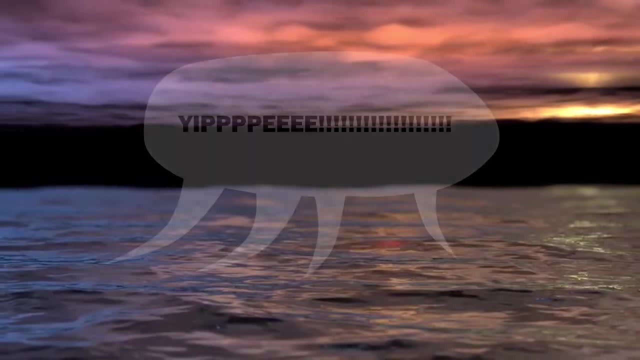 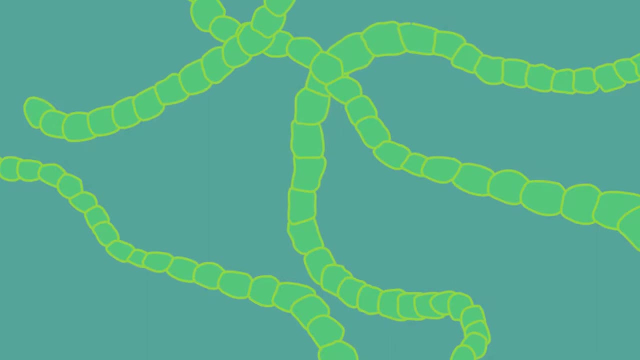 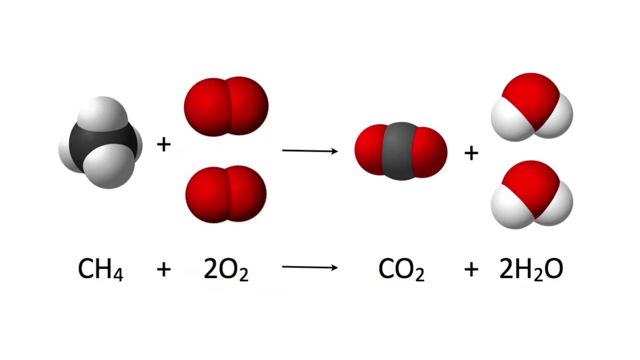 phosphorus into the oceans, allowing microorganisms to flourish. Oxygen-producing cyanobacteria had either recently evolved and radiated or had a much increased presence thanks to the nutrient flux. Their oxygen waste product reacted with this methane to form CO2 and water. Although CO2 is a greenhouse gas, it is 30 times less potent than methane and 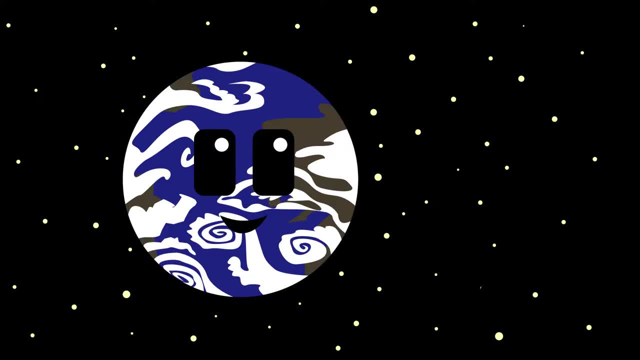 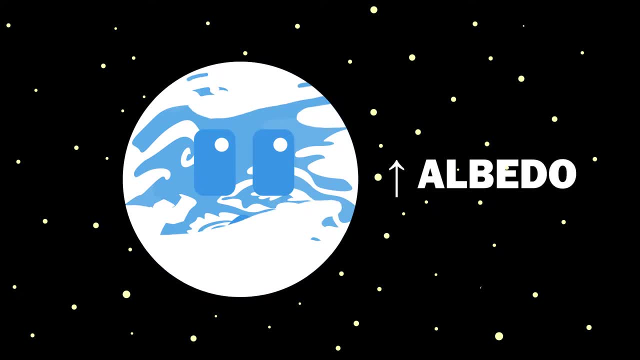 a lot less potent at trapping heat than methane. Hence the earth's temperature began to drop, and as ice crept from the poles, the earth's albedo began to rise. Instead of absorbing heat, the expanding white surface over the earth reflected it. The result was a runaway. 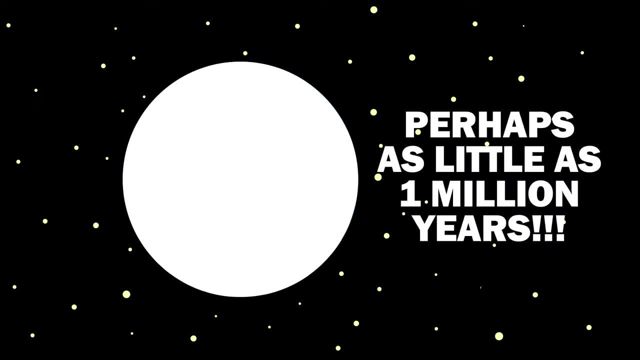 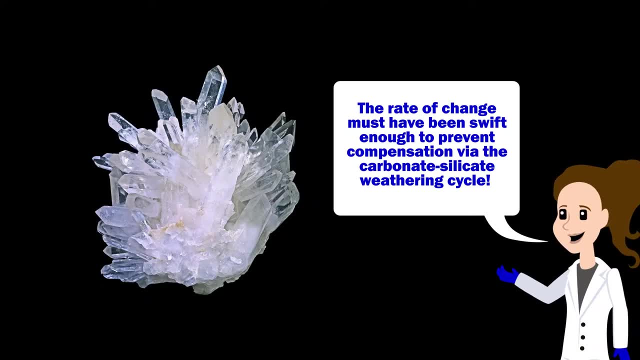 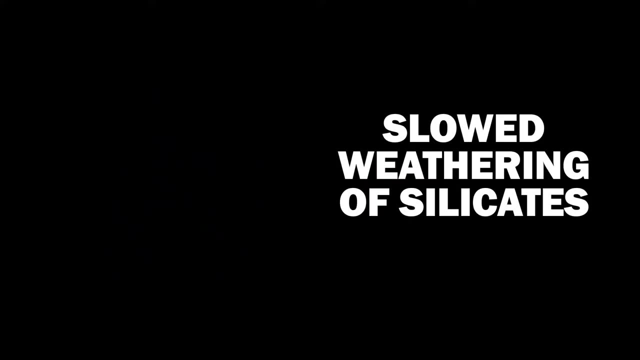 cooling effect, triggering global glaciation in perhaps as little as a million years. The rate of this change must have been swift enough to prevent compensation via the carbonate-silicate-damage scheme weathering cycle. Over a longer time span, cooling would have slowed the weathering of silicates and